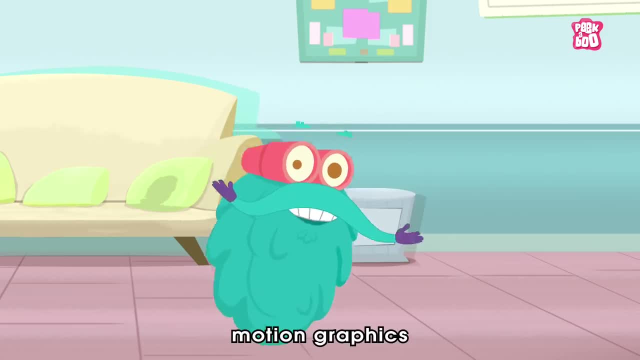 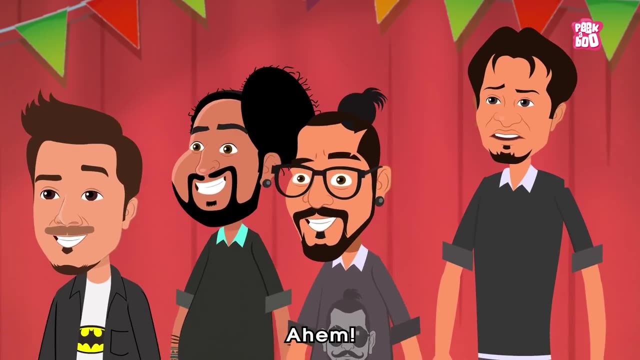 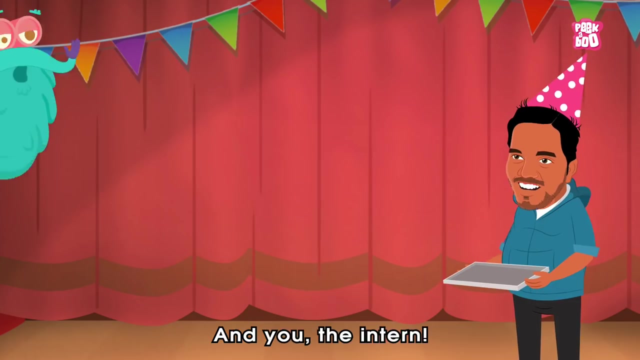 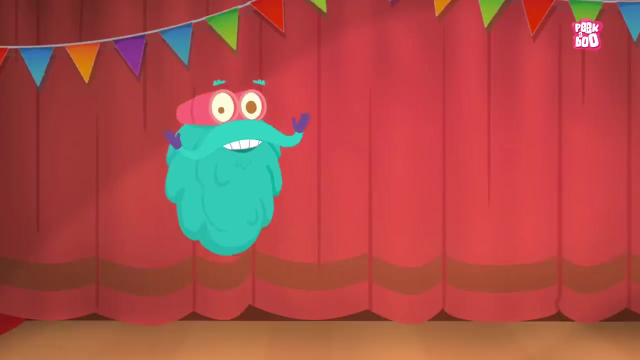 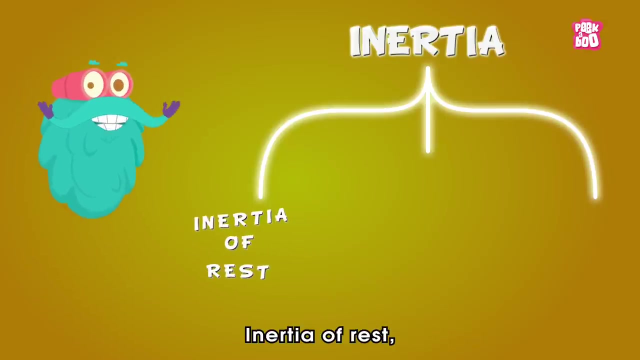 with the help of some cool animated motion graphics Animators. get back to your work, please, And you, the intern, bring some cold coffee for me. Anyways, Inertia can be classified into three categories, that is, Inertia of Rest. 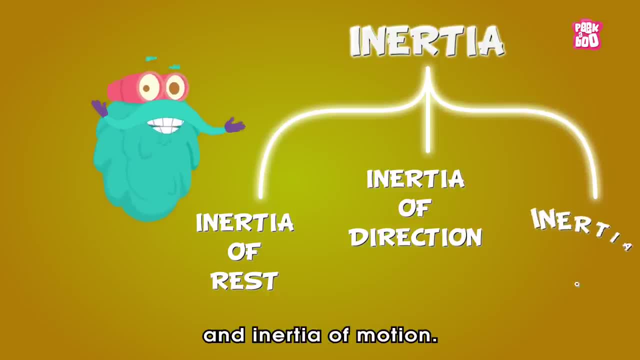 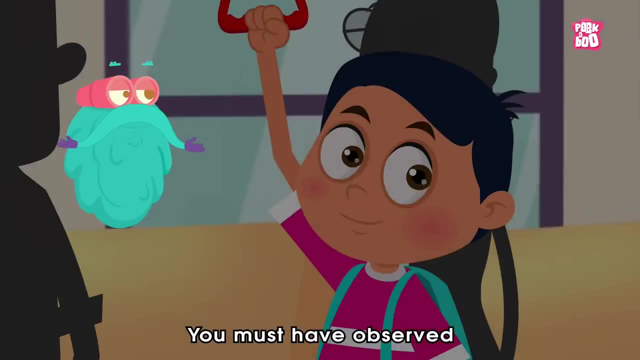 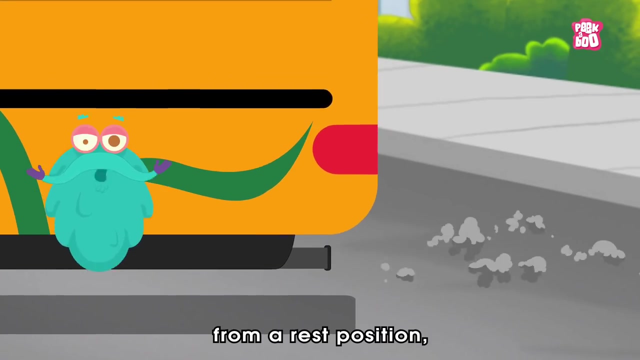 Inertia of Direction and Inertia of Motion. Here is how we experience Inertia in our day to day lives. You must have observed while travelling by the school bus. as soon as the bus starts moving from a rest position, we feel a sudden jerk. 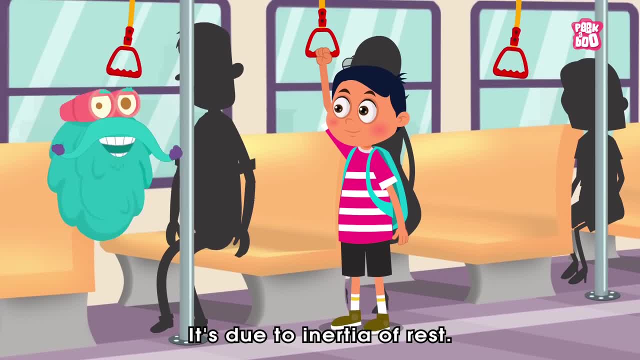 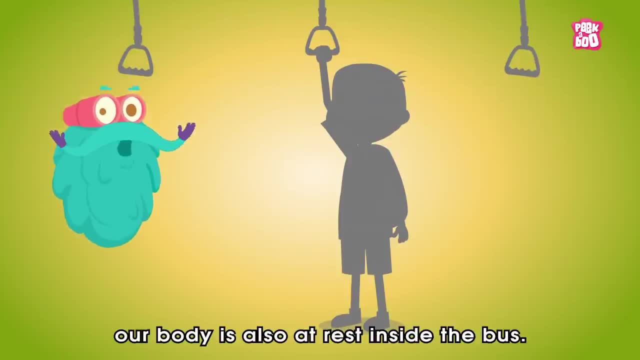 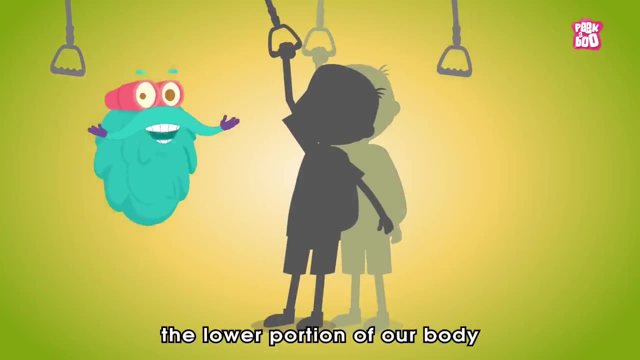 And why is that? It's due to inertia of rest. Yes, when the bus is at rest, our body is also at rest inside the bus. As the bus is put into motion, the lower portion of our body, which is in contact with the bus, acquires velocity. 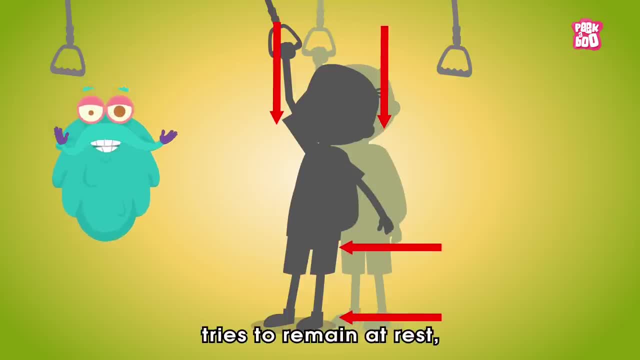 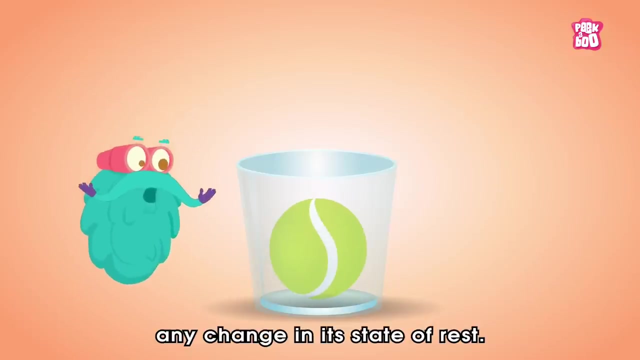 But the upper part of the body tries to remain at rest, making us fall back a bit Due to the phenomenon called Inertia of Rest. That is a tendency of a body to resist any change in its state of rest. And once you are inside the bus, 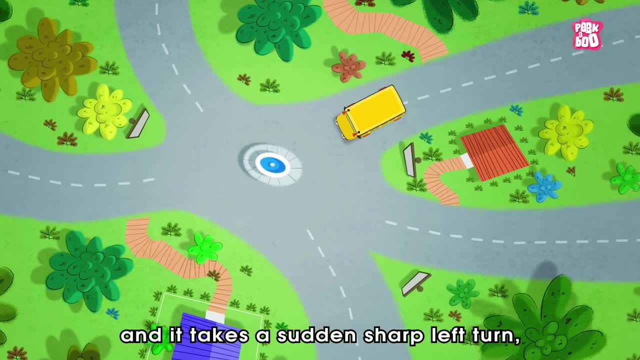 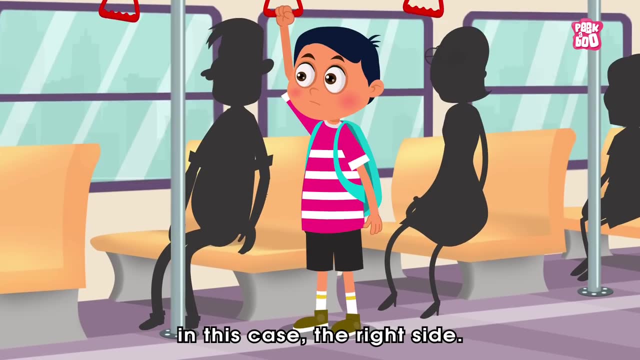 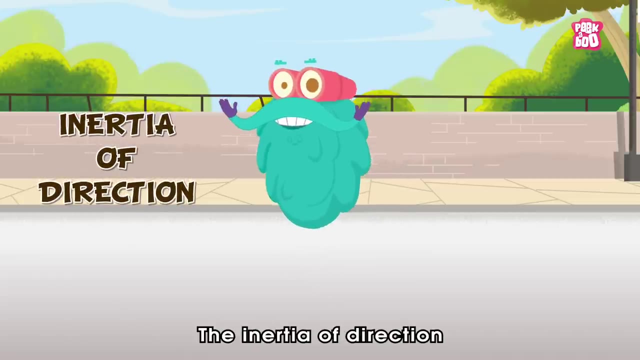 halfway to the school and it takes a sudden sharp left turn, you will feel your body tilting towards the opposite direction, in this case the right side, And this is due to Inertia of Direction. The inertia of direction is a tendency of a body or object. 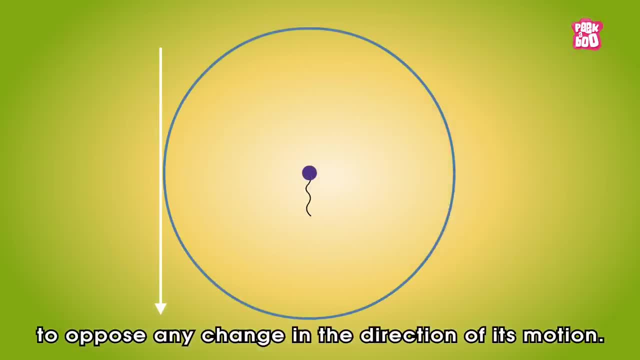 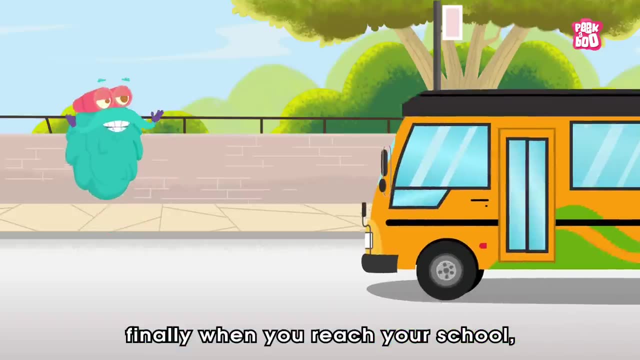 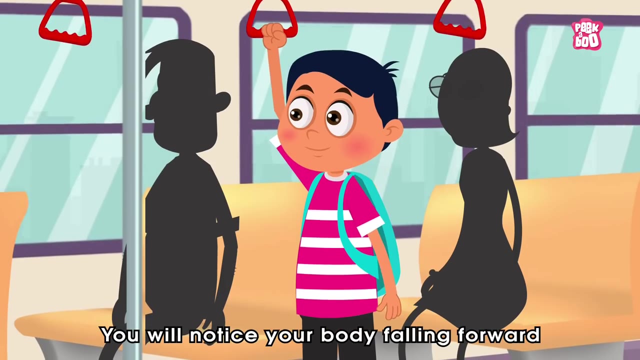 to oppose any change in the direction of its motion And after tossing and turning left and right. finally, when you reach your school and the moving bus suddenly stops by applying brakes, you will notice your body falling forward due to inertia of motion. 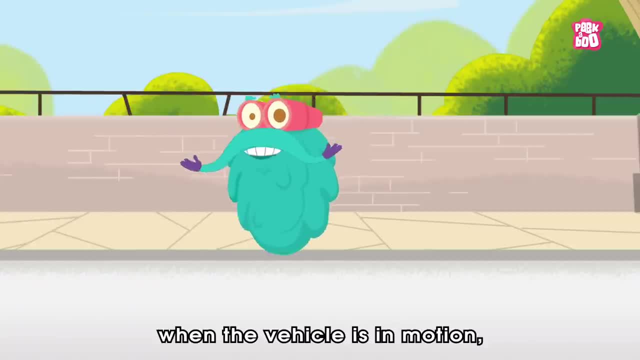 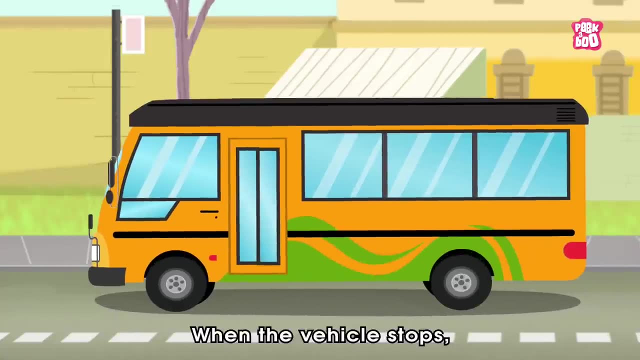 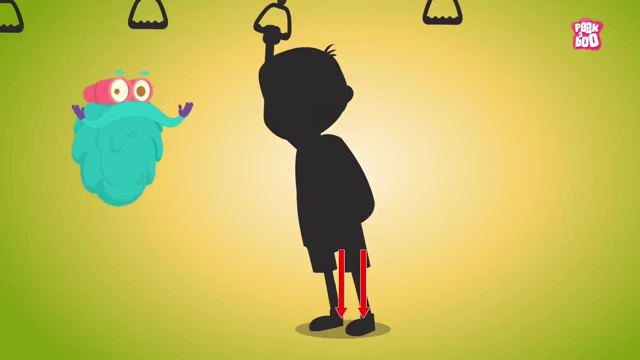 And that is because, when the vehicle is in motion, our body inside the bus is also in motion along with it. When the vehicle stops, the lower portion of our body, which is in contact with the vehicle, comes to rest, But the upper part tries to retain the state of motion. 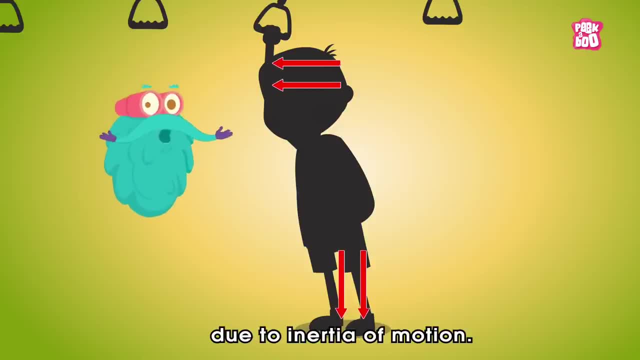 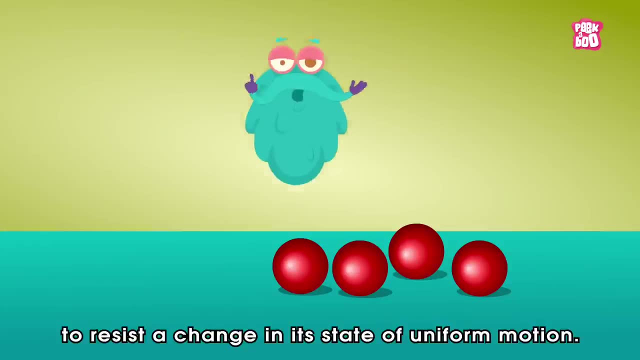 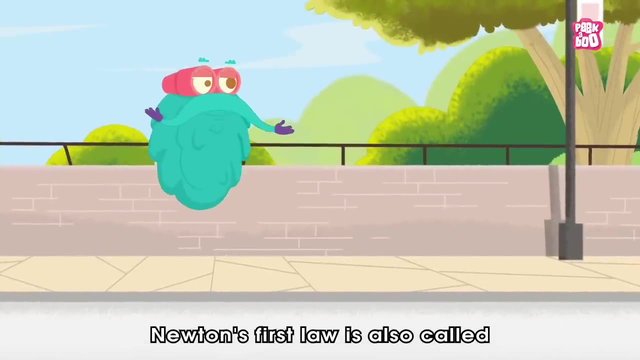 and falls forward due to inertia of motion. Inertia of motion is a tendency of a body to resist a change in its state of uniform motion, And this is the reason Newton's first law is also called Law of Inertia. It's Trivia Time. 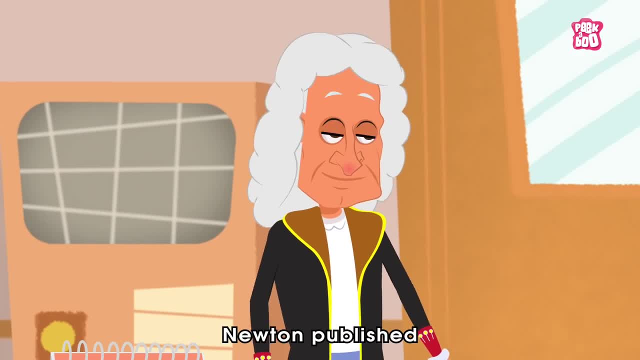 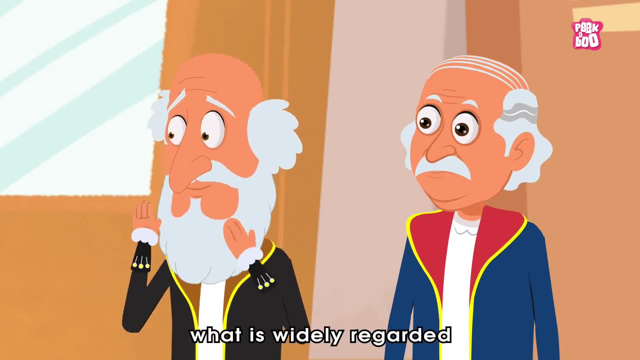 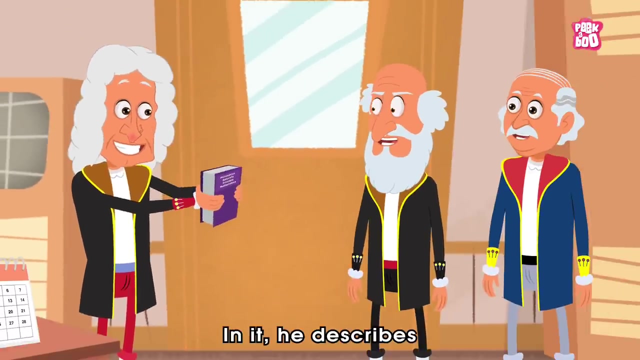 Did you know? in 1687, Newton published Philosophiae Naturalis, Principia Mathematica, what is widely regarded to be one of the important books in the history of science. In it, he describes universal gravitation and the three laws of motion. 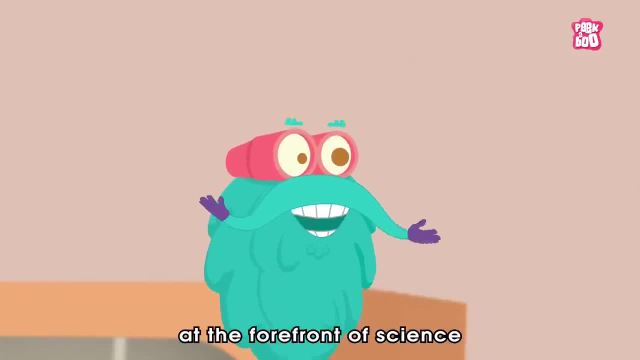 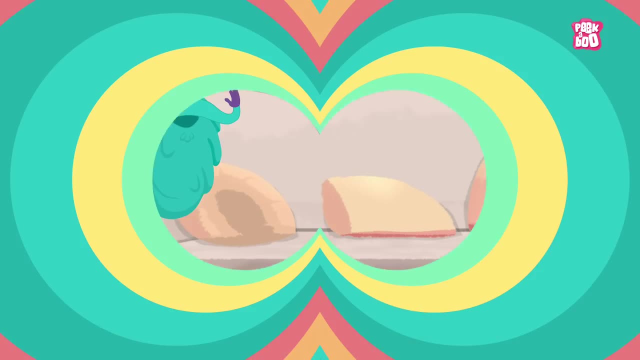 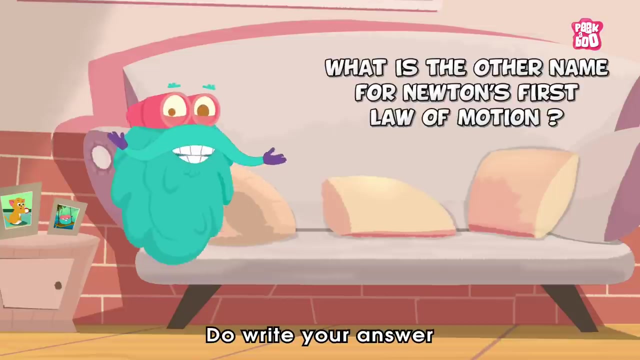 concepts that remained at the forefront of science for centuries. after It's Question Time, Today's question is: what is the other name for Newton's first law of motion? Do write your answer In the comment section below and hit the like and subscribe button if you haven't yet. 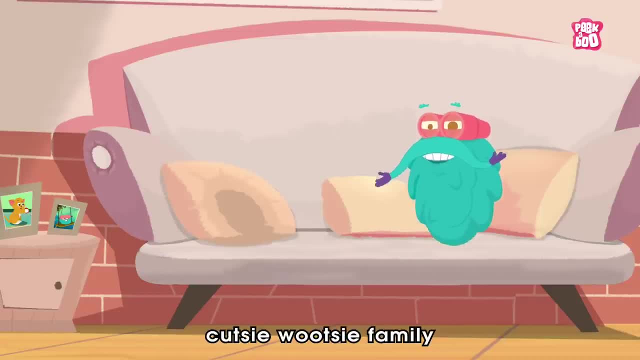 to be a part of the Peekaboo Kids' cutesy-feutesy family and get a chance to get it featured by the end of our videos. So here are the winners of the previous episode. Hope you enjoyed today's episode. 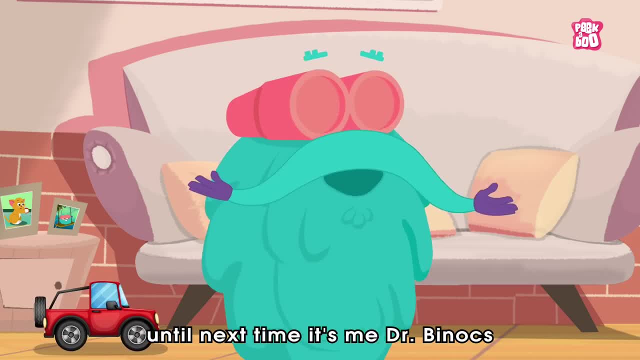 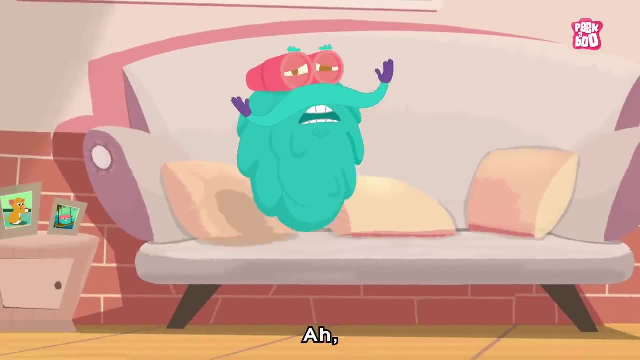 Until next time, it's me, Dr Binox, Zooming Out. See you in the next episode. Ah, never mind. 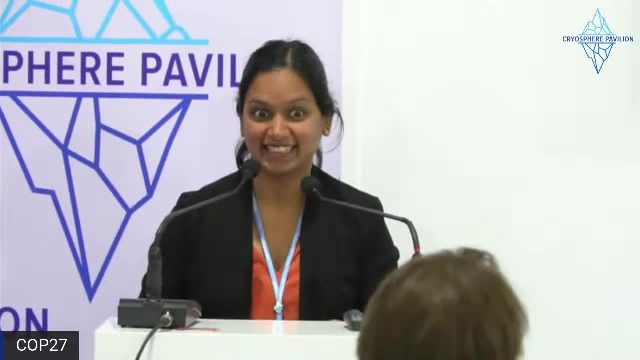 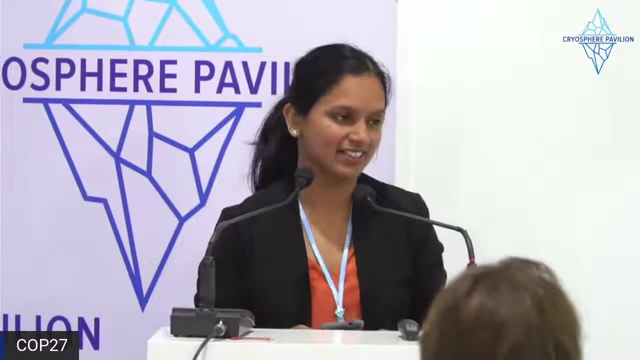 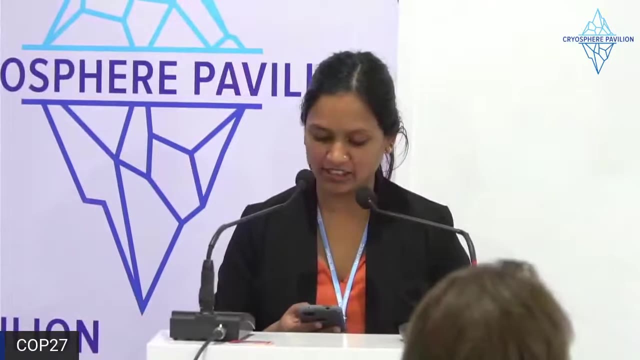 At Concordia University in Montreal, Canada, studying how Arctic bacteria are changing and evolving with climate change, And I'm really happy to be moderating this next session. So welcome to permafrost day. This is a whole day program where we'll be covering the local to.